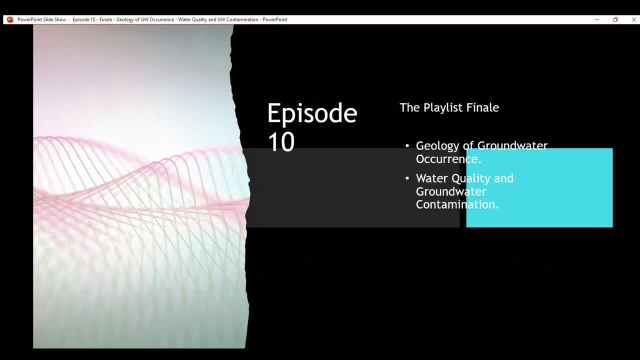 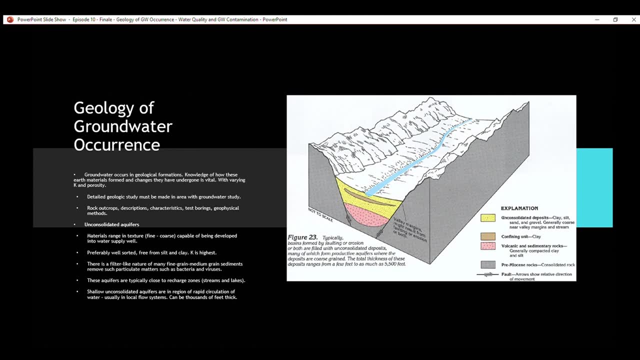 So Geology of Groundwater Occurrence. Groundwater occurs in geological formations. Knowledge of how these earth materials formed and changes they have undergone is vital because they have varying hydraulic conductivity and porosity. A detailed geologic study must be made in an area with groundwater, with a groundwater study. 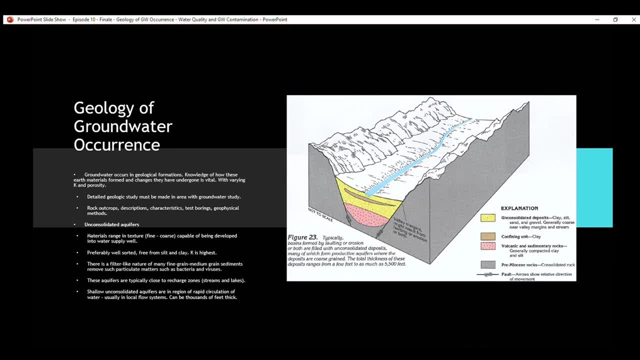 You study the rock outcrops, You describe the rocks, their characteristics, You take borings, You use geophysics And then you have probably the most common aquifer, which is the unconsolidated aquifer, in terms of extracting water out of. 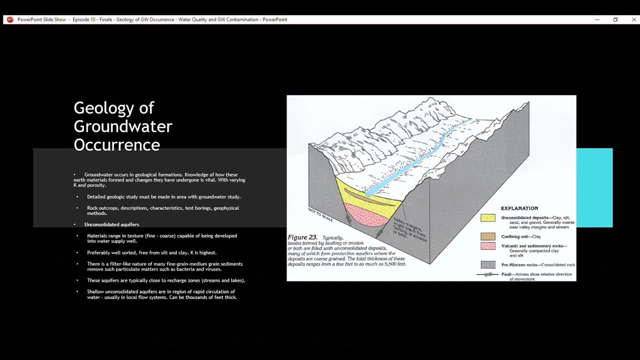 You have materials that range in texture from fine to coarse, capable of being developed into a water supply well, Preferably well sorted and free from silt and clay, because they fill up the spaces between grains. Hydraulic conductivity is highest in, say, a well sorted ground. 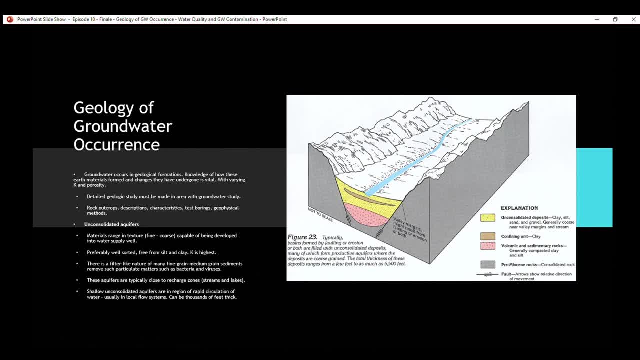 Well sorted gravel or well sorted sand. There is a filter, like nature of many fine grain, medium grain sediments that remove such particulate matters such as bacteria and viruses. And I know here in El Paso they use, they recharge the aquifer at the mountain and it travels. 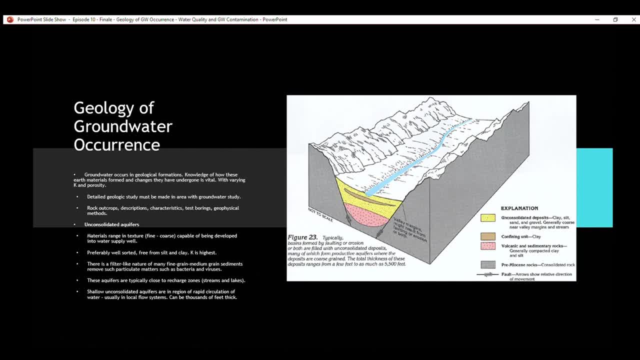 Obviously it's a, it's a regional, It's a large scale groundwater flow. So they They use, they basically inject. It's called injection wells. They inject into injection wells used water and that water will naturally become felt filtered through time. 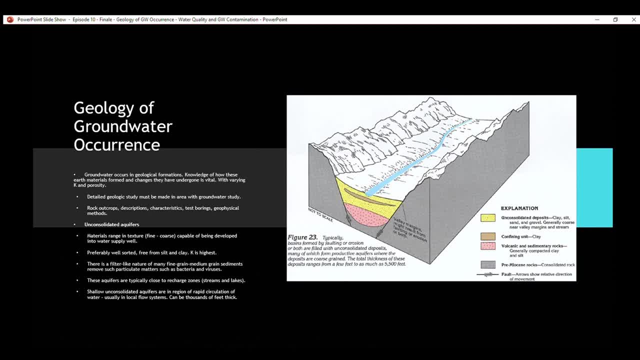 So that's what that's talking about And that's one positive about unconsolidated aquifers is: the water is typically very clean And these aquifers are typically close to recharge zones. as you can see in this photo, You have a recharge zones at a stream or at a lake, and shallow unconsolidated aquifers are in a region of rapid circulation of water, which is usually in local flow systems. 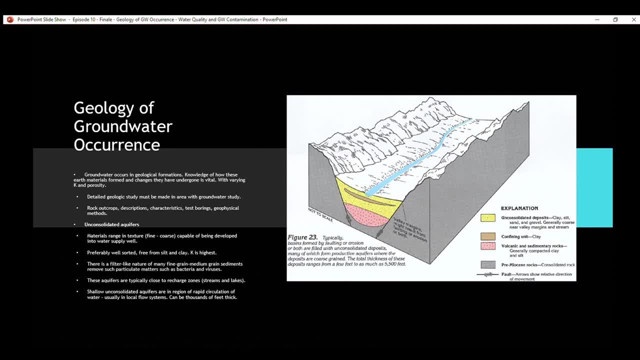 So the groundwater doesn't take a lot of time between recharge and discharge. So if the water enters here, let's say this is a fault. If it enters here, The water doesn't take a lot of time to discharge at the stream, And these aquifers can be thousands of feet thick. 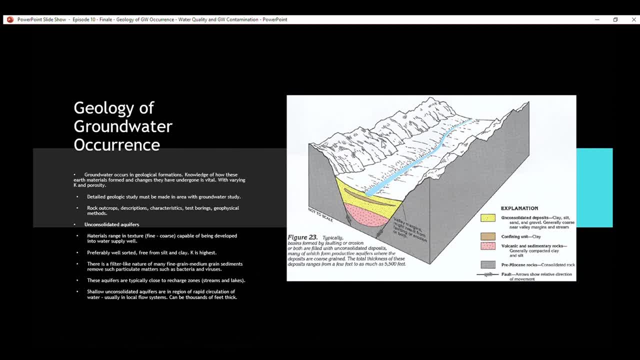 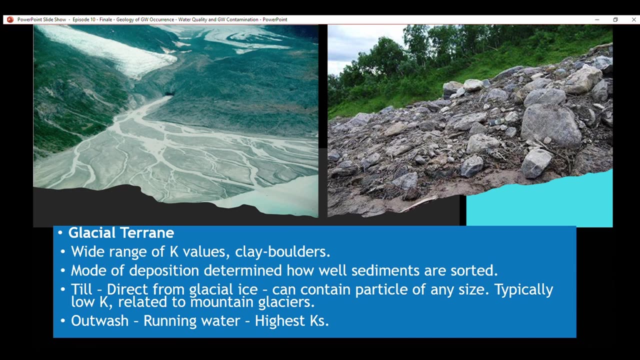 So, in terms of glacial terrain, which obviously I have no experience dealing with, but I will briefly go over it- You have a wide range of hydraulic conductivity values. It can vary from clay to boulders. Your motor deposition is determined by how well it's. 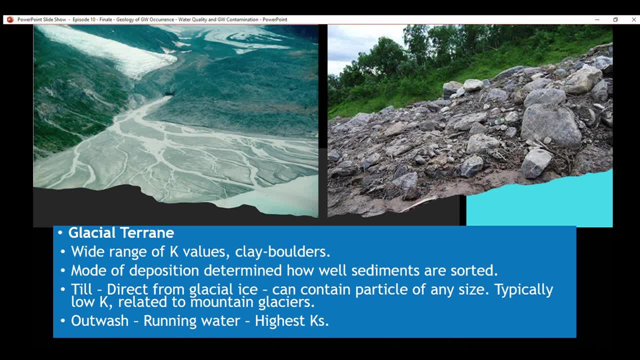 the sediments are sorted and a till. it's directly from glacial ice. it can contain particles of any size and typically has low hydraulic conductivity and it's related to mountain glaciers. i know that till can have clay or it can have boulders and it's poorly sorted. you're going to have low. 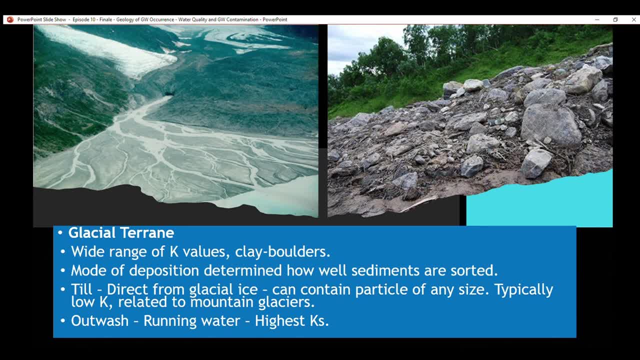 hydraulic conductivities. and then in terms of outwash- glacial outwash- it's deposited by running water, so you'll have higher k's because it's it's better sorted. it's not necessarily great sorting because you still have clays and silts, but it'll have higher k's than the till. 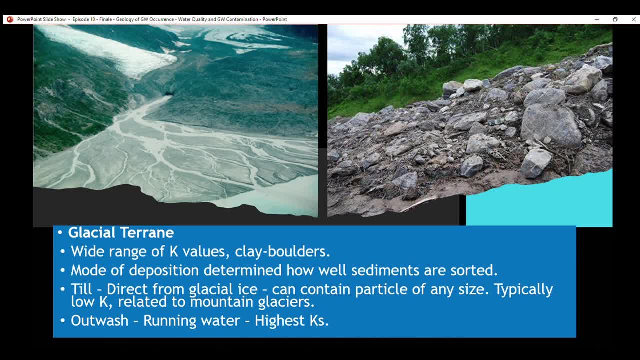 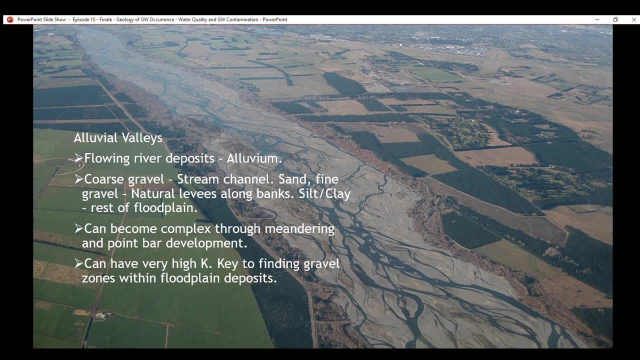 and in terms of alluvial valleys, obviously flowing river deposits are alluvium, coarse gravel represents a stream channel and sand, fine gravel are natural levees along the banks. so you and- well, actually this is meandering, so it's going to complicate things, but this is your floodplain on this, uh, on this stream most, yeah, river valley, whatever. 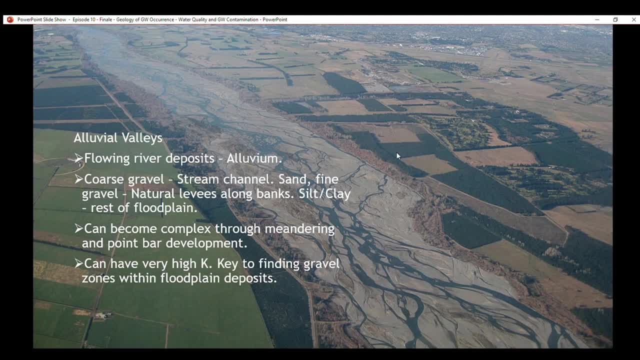 um, coarse stream would represent the, the current stream. so this, you just follow this. you probably find your coarse gravels and then your natural levees are somewhere right here. maybe right here when you have meandering at complex, complex, but, um, so you're fine gravel and sands, you're going to find that, the natural levees, and then 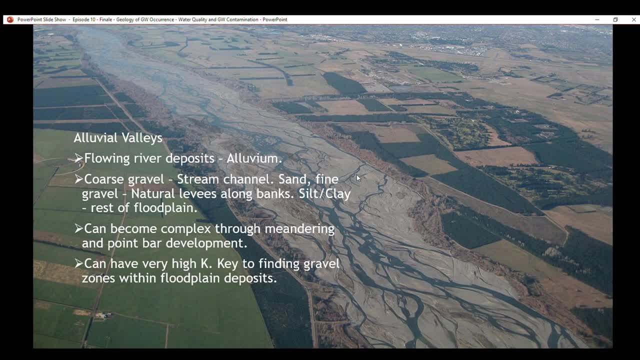 silt and clays are in the floodplain. it can become very complicated through meandering and point bar development. it can have very high k hydraulic conductivity and key. the key is to find gravel zones within floodplain deposits because that's going to be the best sorted. 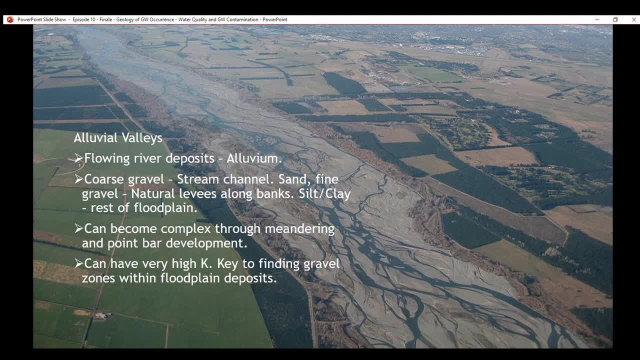 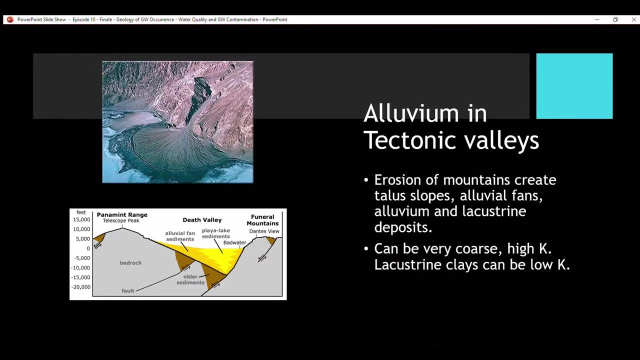 material in a alluvium valley. so alluvium and tectonic valleys, we're talking about pretty much alluvial fans. but the erosion of mountains create talus, slopes, alluvial fans, alluvium and lacustrine deposits. it can be very 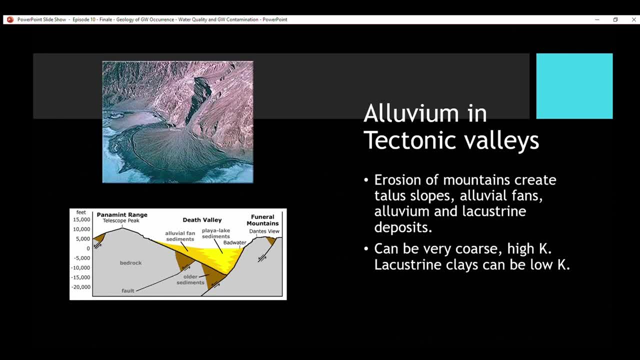 coarse. uh have high, high, uh sorry, have high hydraulic conductivity. uh, lacustrine clays, which is a late clay, can be low k and this picture represents an alluvial valley alluvial fan. it's a nice looking alluvial fan and these would have typically have. uh, you know. 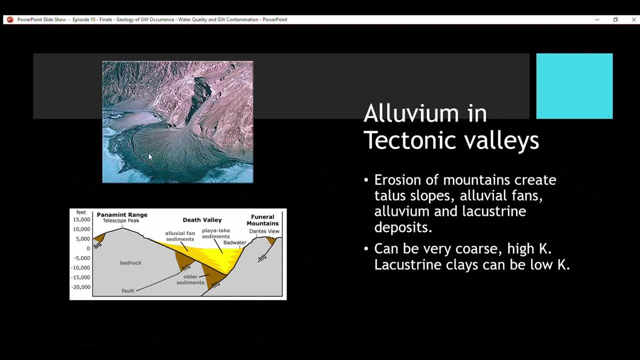 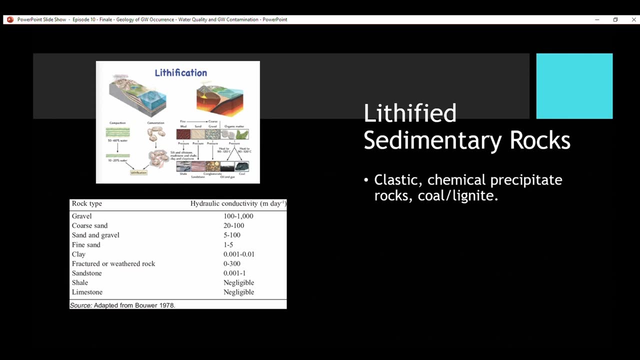 decently high k because, uh, it's pretty well sorted. it's sorted by water, running water, um going down the slopes of a mountain. so in terms of lith- and we'll dig deeper into this later on in this, uh this presentation- but lithified sedimentary rocks, clastic, uh chemical precipitate rocks, uh coal and 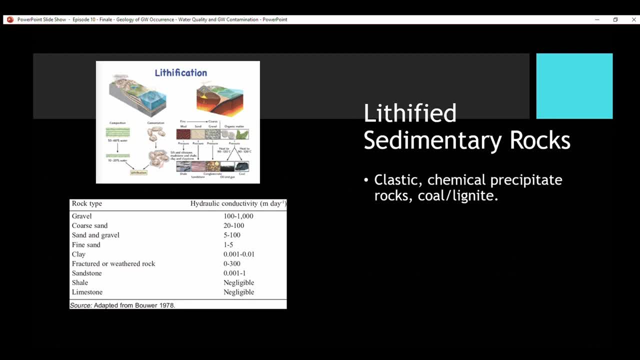 lignite and this gives you a little table showing. basically, from here on uh, sandstone is going to have the highest k, shell and limestone are going to be negligible. limestone can be dependent on fracturing. shell is typically very low k, um. horizontally it has good k, but vertically like uh. like we said in a, 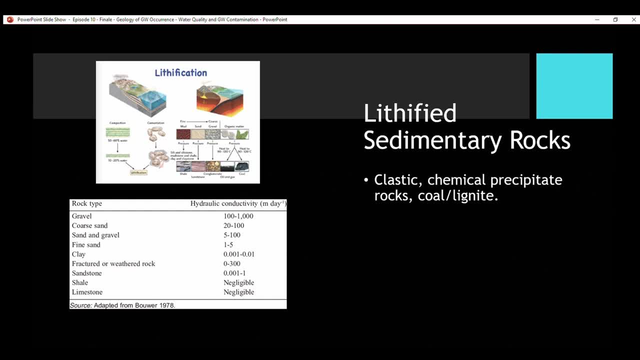 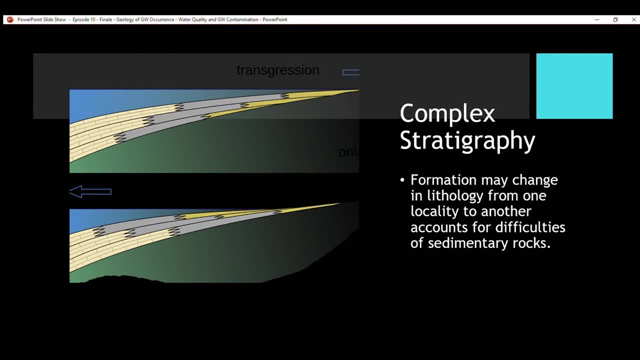 previous episode. uh, so complex stratigraphy can complicate, um the uh occurrence of the aquifers. so this is showing. uh, let's see, take a cross section of this right here. that is a transgression and then this one's a regression of: uh, if you're into that stratigraphy, 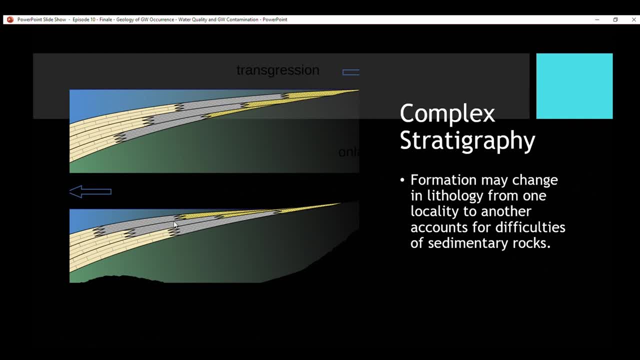 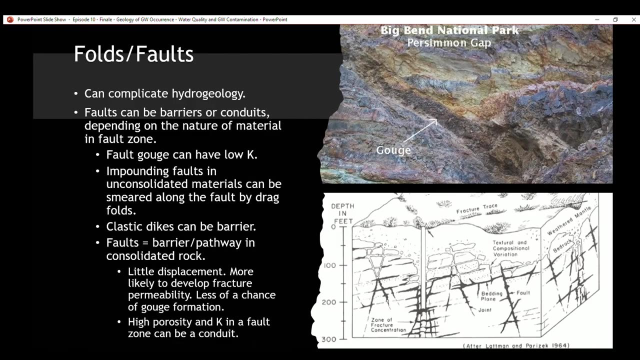 anyways, a formation may change in lithology from one locality to another, which accounts for difficulties of uh interpreting sedimentary rocks. for aquifer development. uh folds and faults can complicate hydrogeology. faults can be barriers or conduits depending on the nature of the material in the fault zone: fault gouge, which is basically ground up rock um created during fault. 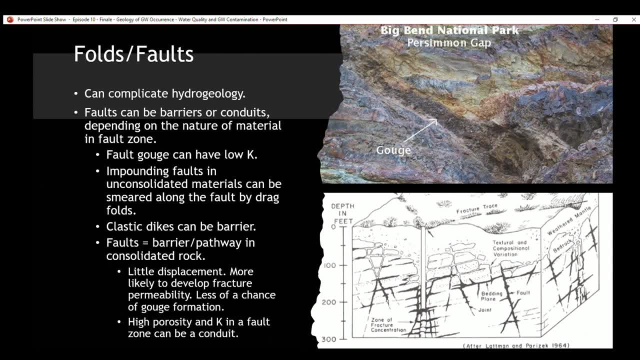 slip uh can have very low k because it's very fine. there's not going to be a lot of pores between the the gouge and here's a good picture of what gouge looks like. this is at big ben national park. i believe this was a reverse fault. 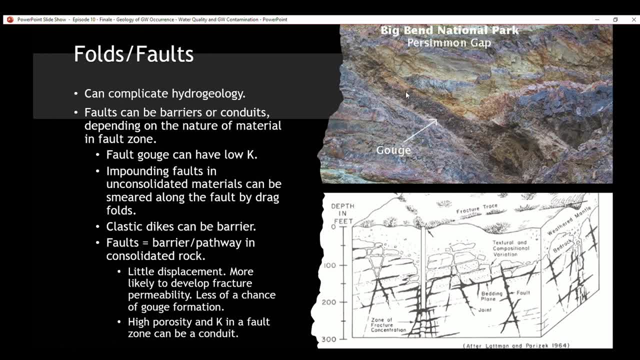 impounding faults and materials can be smeared along the fault by drag folds and a clastic dike can be considered a barrier. faults equals either a barrier or pathway in consolidated rock: little displacement, more likely to develop fracture, permeability and less of a chance of gouge formation. 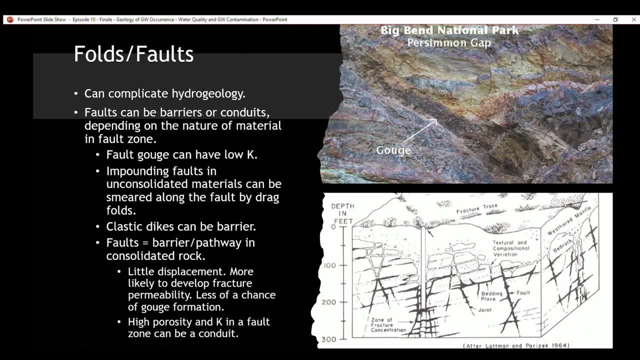 and high porosity and hydraulic conductivity in a fault zone can be a conduit to uh, to groundwater recharge or discharge, either one, and then this picture just kind of shows: uh, basically a limestone, uh environment, and uh you have these fractures that can become either conduits or they can be barriers, depending on if they've been mineralized or not. so folding? well, that that font's small, okay, folding can create confinement. so in fact, when i say folding, I'm talking about found engaged or confined to non-contaminated rock. And if you create a bond to the surface, where there is less water in it, the ice that's inside can be formed, and if the ice is less, there isn't as much ice in it and thearring inside can leave more of an impact to the surface. 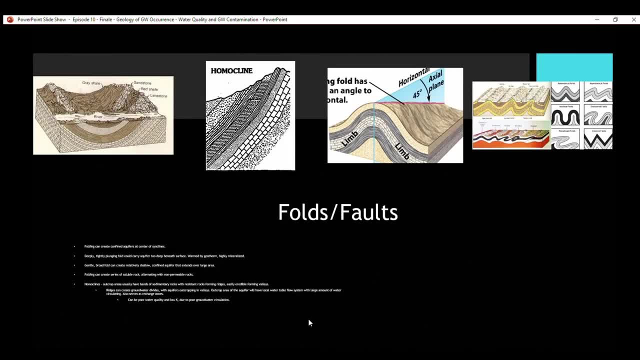 So, now that your having some involve your work, there might be some form of friction between the rocks. okay, folding can create confined aquifers at the center of, uh, synclines, which is, let's see, syncline. yeah, okay, syncline. syncline is over here on the left. um, actually, let me make sure. 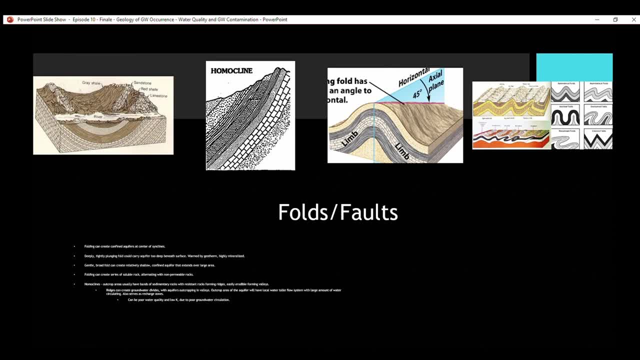 yeah, okay, yeah, it's been a while. um. so a deeply, tightly plunging fold can carry an aquifer too deep beneath the surface and it can be warmed by the geotherm and highly mineralized gentle. broad folds can create relatively shallow, confined aquifers that extend over a large area. 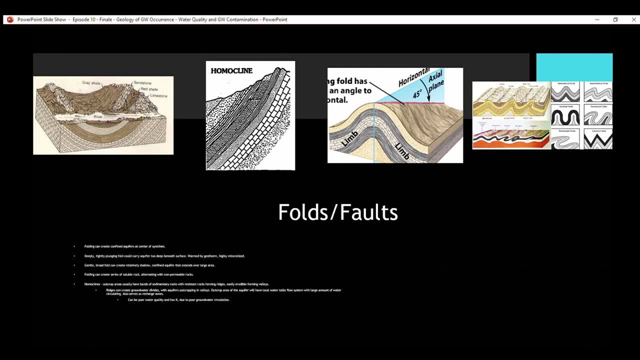 folding can create a series of soluble rock alternating with non-permeable rock, so like a sandstone and a shale, alternating homoclines, which outcrop areas usually have bands of sediment rock with resistant rocks forming ridges, easily eroding, easily erodible, and they can form valleys. 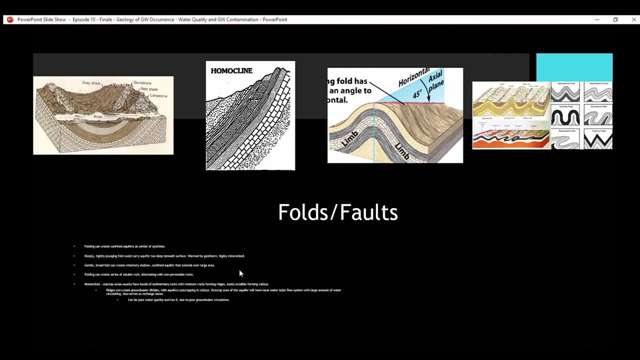 so this is a limestone that looks like a sandstone shell. right here you have a valley form like these, where the shells are, and that would be, that would be the values that they're talking about right there. um, let's see, and so the ridges can create. 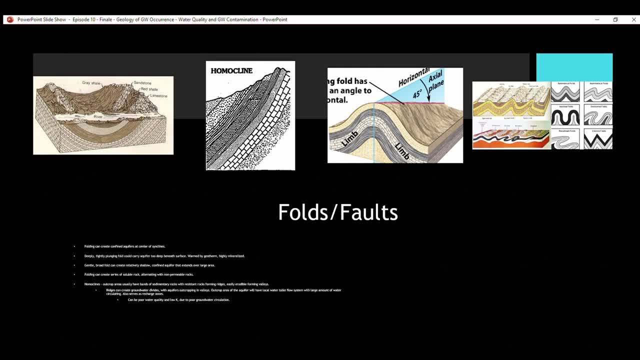 outcrop areas and they can create ground water divides with aquifers outcropping the valleys. an outcrop area of the aquifer will have a local water. water table flow system with a large amount of water circulating also serves as a recharge zone. um, so like we were talking about, shale is. 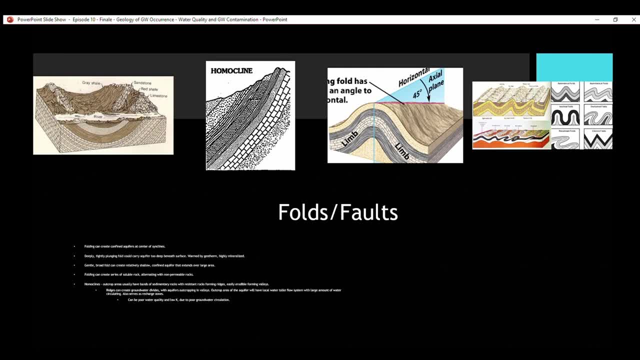 going to be easily erodible, but water most likely isn't traveling in and whereas you have a sandstone right here, that's going to be hot, more permeable, more porosity. so water is going to be recharged there. depending on the fracture characteristics of the limestone, maybe it can. 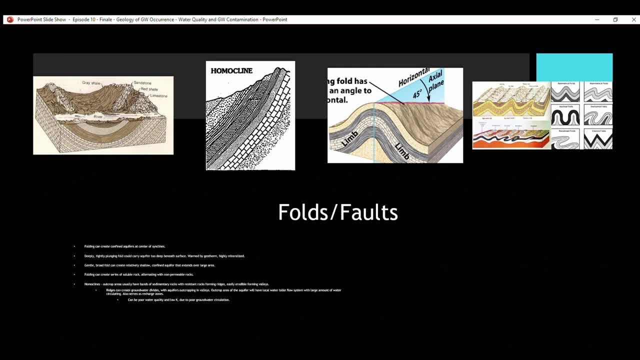 flow into the limestone, but most likely it's the sandstones and maybe this looks, maybe like it could be a conglomerate, which would be a higher k and the water quality could be poor and have locate due to poor groundwater circulation. homocline is just one. 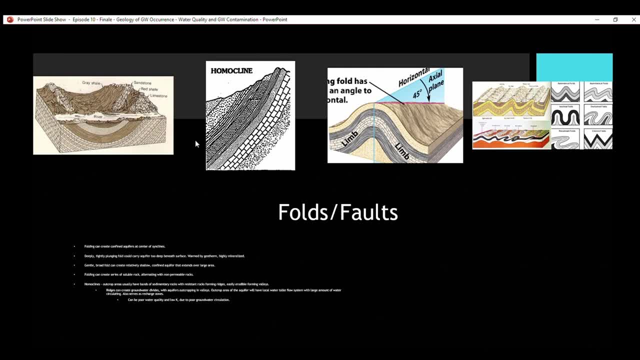 uh, basically one limb of a fold. so, um, where is it going into the surface? probably deep and it's not discharging anywhere, so it's going to have poor groundwater circulation. that's what that's talking about. okay, so classic sedimentary rocks: hydraulic conductivity based on the primary. 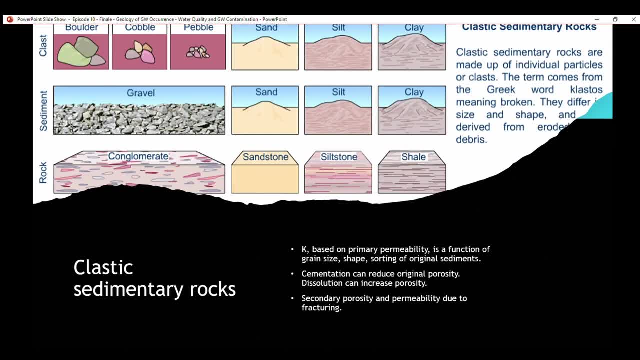 permeability is a function of the grain size, shape, sorting of the original sediments: cementation can reduce original porosity and dissolution can increase porosity. secondary porosity and permeability would be due to fracturing. and if you guys don't remember what primary permeability is, primary permeability is permeability. 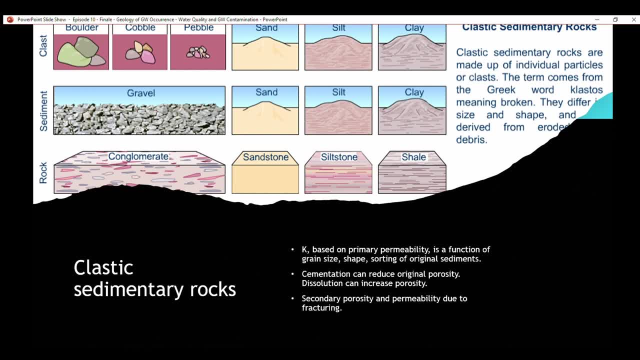 was there when the rock formed, and then secondary is everything that happened after formation. so a fracture of a sandstone or a limestone is considered secondary in terms of carbonate. rocks of a limestone or a dullo stone is variable. a crystalline limestone will have very low porosity. 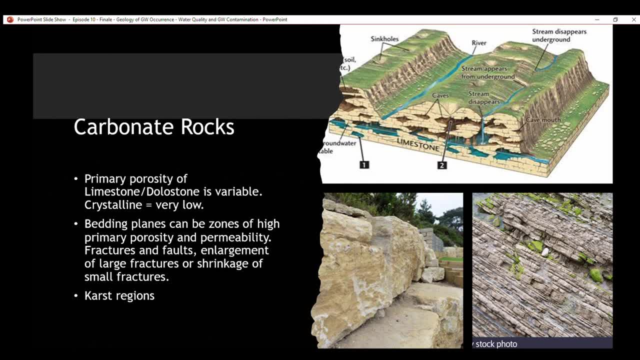 bedding planes, as you can see in this beautiful outcrop right here. these bedding planes right here can be zones of high primary porosity and permeability. fractures and faults, enlargement of large fractures or shrinkage of small fractures can affect the porosity of a limestone and then 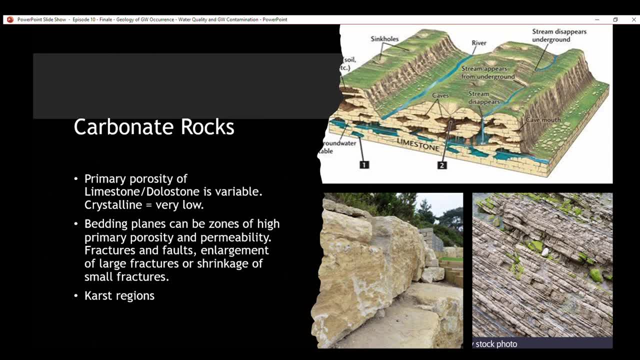 obviously you have your karst regions, which can create an increase in porosity. in a limestone environment, a karst is it's called a karst region. dissolution due to, like a mix of hydrochloric acid and water, can dissolve this limestone and create these caves and obviously water can travel through. 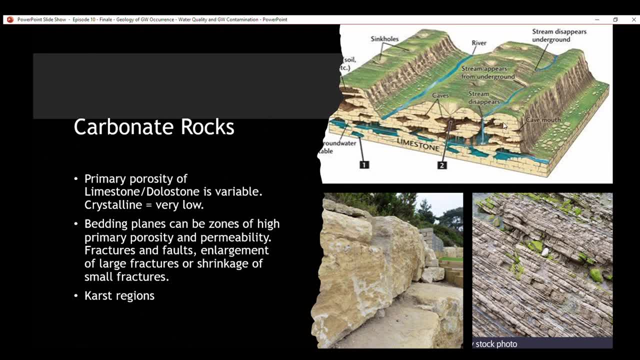 those, and it would be very helpful to study karst geomorphology so you can understand why a stream would disappear here and then reappear and how all this happens. it's- it's pretty interesting- groundwater in desert areas. so a desert area is low precipitation- less than 10 inches annually. 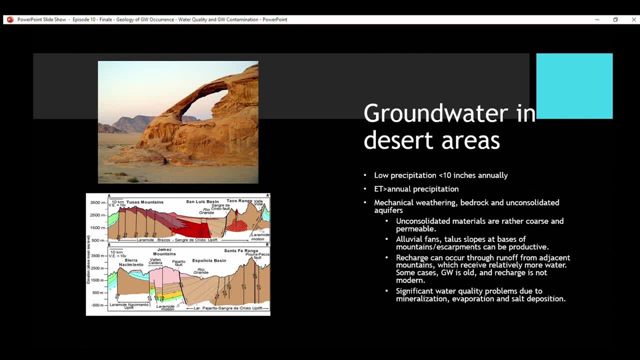 evapotranspiration is greater than the annual precipitation. mechanical weathering is very common. it it out does chemical weathering. because chemical weathering is more prevalent in an environment like a tropical region, a lot of dissolution going on, bedrock and unconsolidated aquifers are common in desert areas. you have unconsolidated materials that are rather coarse. 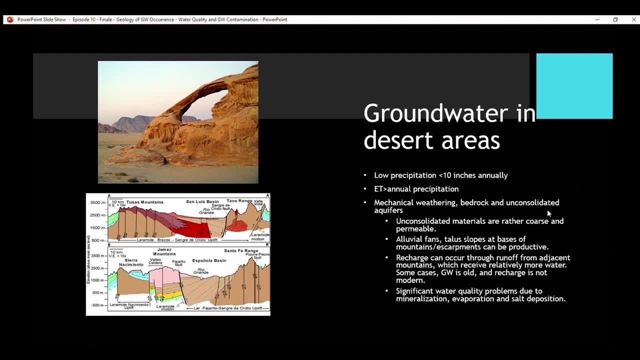 and permeable. you have your alluvial fans, talus slopes, at the bases of mountains or escarpments, which can be productive. recharge can occur through runoff from adjacent mountains which receive relatively more water. some cases the groundwater is old and recharge is not modern, which would be the case in a regional groundwater flow regime. significant water quality. 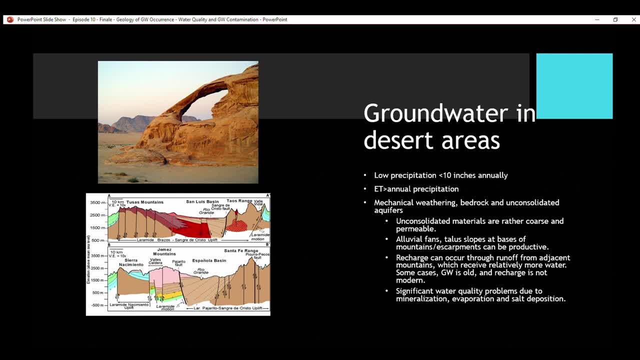 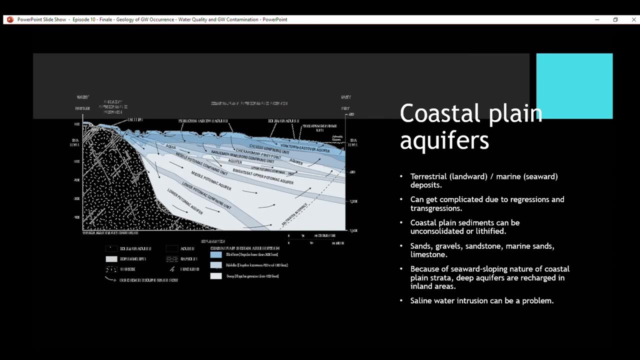 problems due to mineralization, evaporation and salt deposition can be prevalent in groundwater desert areas, so coastal, plain aquifers, terrestrial, which is landward deposits, and marine, seaward deposits. it can be complicated due to regressions and transgressions, like we talked about in a 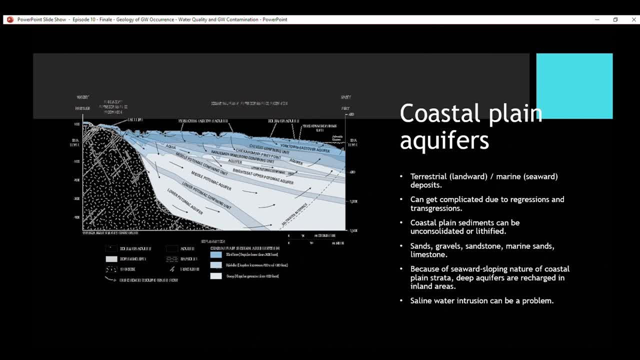 previous slide. coastal plain sediments can be unconsolidated or lithified sands. gravel sandstone, marine sands and limestones are present. you can also include some shell. because of seaward sloping nature of the coastal plain strata, deep aquifers are recharged in inland areas and one issue that you have in these aquifers is saline. 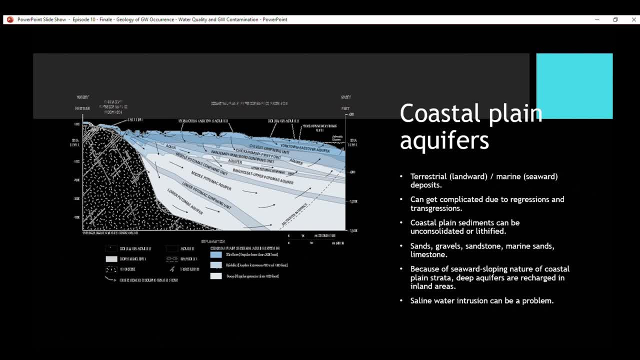 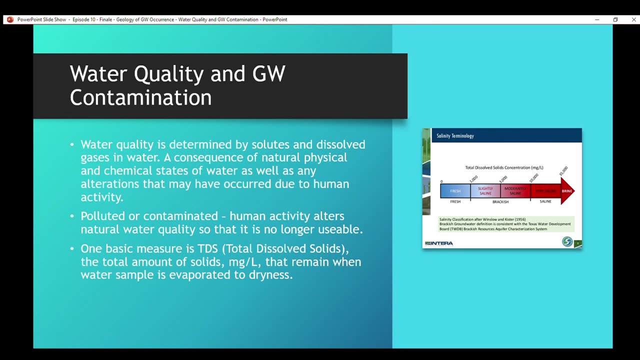 water intrusion. obviously seawater intrudes into the aquifer, which is fresh water, and basically makes that water undrinkable. so water quality and groundwater contamination. water quality is determined by solutes and dissolved gases in water as a consequence of natural, physical and chemical states of water, as well as any 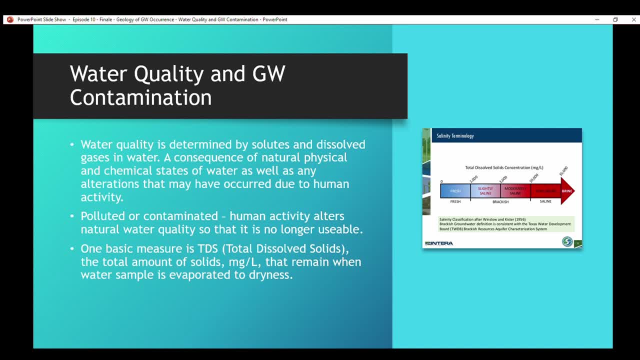 alterations that may have occurred due to human activity and so polluted or contaminated. human activity alters the natural water quality so that it is no longer usable. one basic measure is TDS, total dissolved solids. the water is the total amount of solutes, milligrams per liter, that remain when water sample is evaporated to dryness, and this is a little chart that shows you. 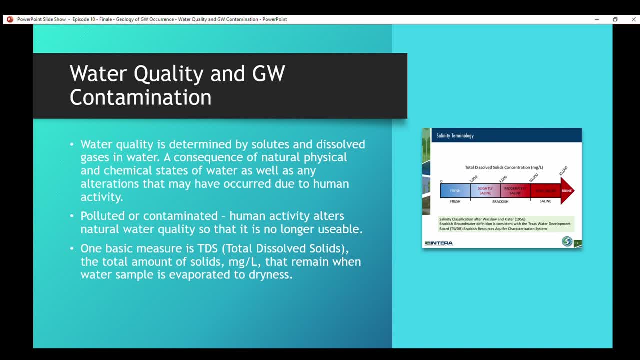 less than 1000 milligrams per liter is considered fresh water, and then anything above that is going to be considered saline, and once you get to this 35000 milligrams per liter, you're in brine. obviously, the water is depending on the state that you live in. 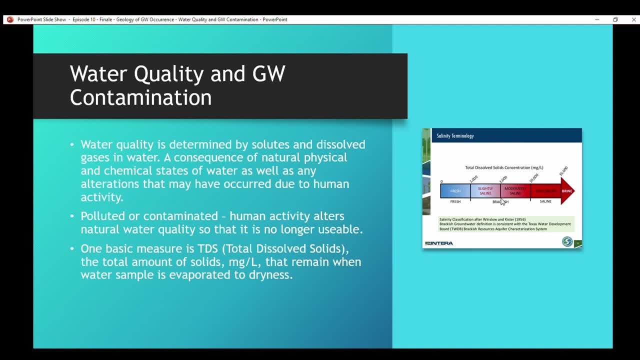 I can pretty much be undrinkable to this point. but it's not just the water that is just being produced, or beingtr鈠 maybe earlier. typically you find this type of water in oil drilling, really, but anywhere that there's been a like a limestone, a previous transgression or regression of what our 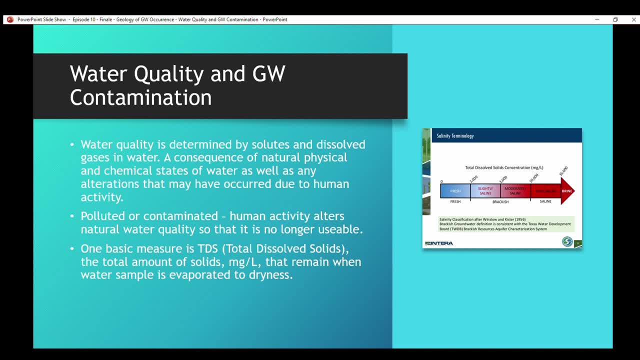 marine sediments, limestones can create. well, not just limestones but also halite. a lot of halite deposition, evaporation from an ocean can create this seawater as that gets buried into the ground. so total dissolved solids, and there's another chart that shows what's acceptable. 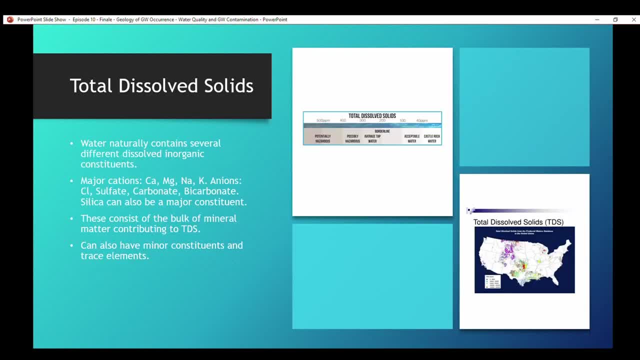 water and this is in ppms. but potentially hazardous and possibly hazardous is anything up to 300 ppms. that's not in milligrams per liter. we'd have to convert that, but anyways. so water naturally contains several different dissolved and inorganic constituents. major cations, which is a positively charged, basically metal, is calcium, magnesium, sodium, potassium and 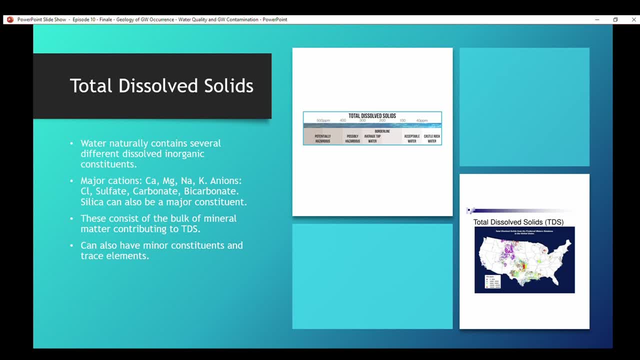 your anions are chloride or chlorine. sulfate carbonate, bicarbonate. silica can also be a major constituent. these consist of the bulk of mineral matter contributing to tds, and you can also have minor constituents and trace elements like copper. dissolved gases can be present in both surface and groundwater, which include 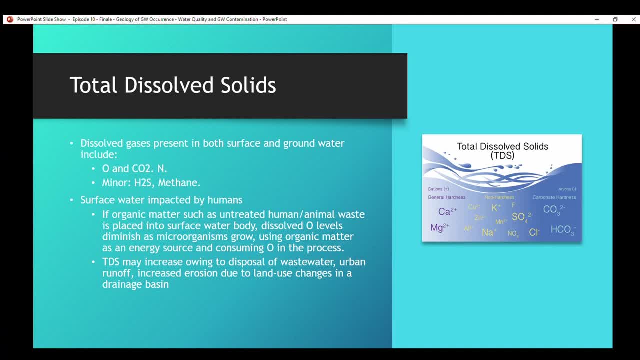 oxygen and carbon dioxide nitrogen, and then, in terms of minor uh constituent gases, would be h2s and methane, which are two really bad ones. um, this chart on the right kind of shows you what contributes the most to general hardness in terms of the cations, and then you have. 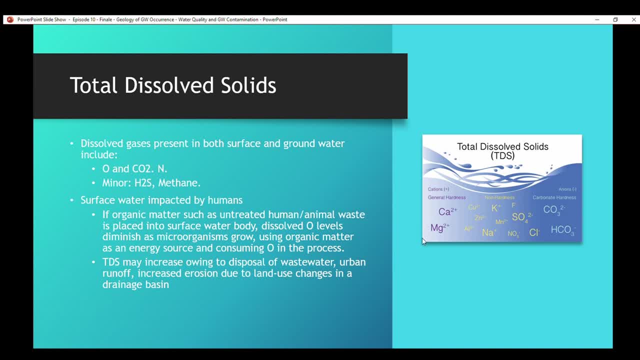 carbonate, hardness contributed by the bicarbonate and the carbonate, and then, according to this, hardness isn't contributed by sulfate, chloride, uh, sodium, manganese, potassium, zinc, aluminum. i don't remember what that is, i think it's just night and what's it called nitrate. anyways, yeah, it's a crash course on chemistry again. 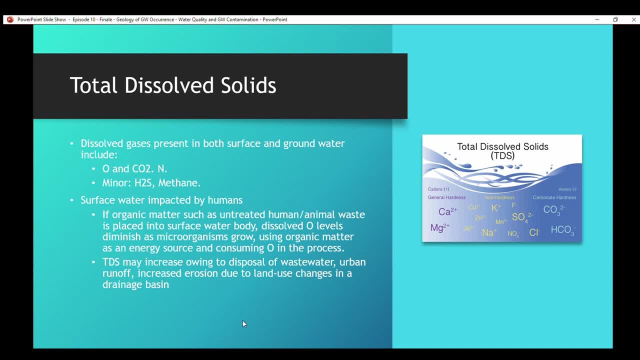 okay, so surface water impacted by humans. if organic matter such as untreated human animal waste is placed in the surface water body such as a, a lake, uh, dissolved oxygen levels diminish as microorganisms grow. they use the organic matter as an energy source and consume oxygen in the process, which kills the animals that are in the uh. 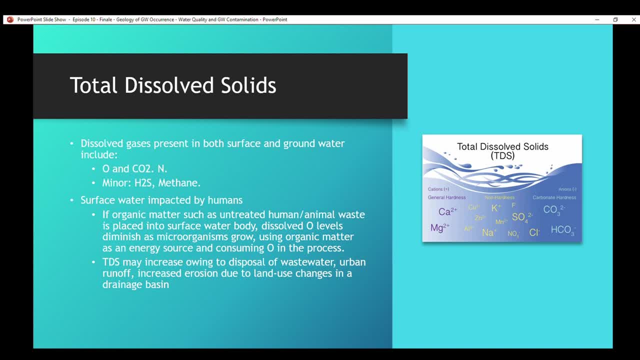 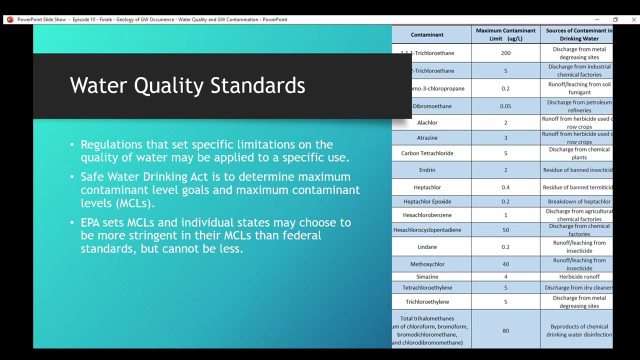 in the water and uh kills the water. really. tds may increase owing to disposal of wastewater, urban runoff, increased erosion due to land use changes in a drainage basin. so your water quality standards? this chart on the right shows you a contaminant, the maximum contaminant limit, which is the mcl, and potential sources of contaminant in drinking water, so triochloroethane. 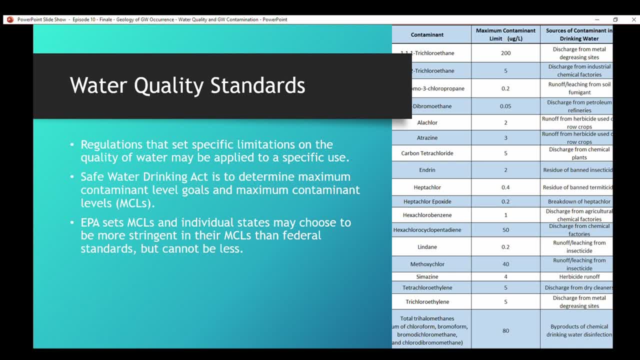 is 200 micrograms per liter and it potentially comes from discharge from metal degreasing sites and you can just run through that herbicide runoff is simosine lindane runoff leaching from insecticide. you know this. these are really bad things, okay. so regulations that set specific. 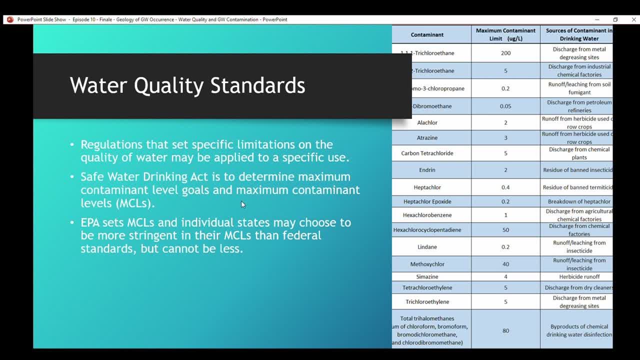 limitations on the quality of water may be applied to a specific use. the safe drink- safe water drinking act is to determine the maximum contaminant level goals and maximum content contaminant levels, mcls. epa sets the mcls and individual states may choose to be more stringent in their mcls than federal standards, but cannot. 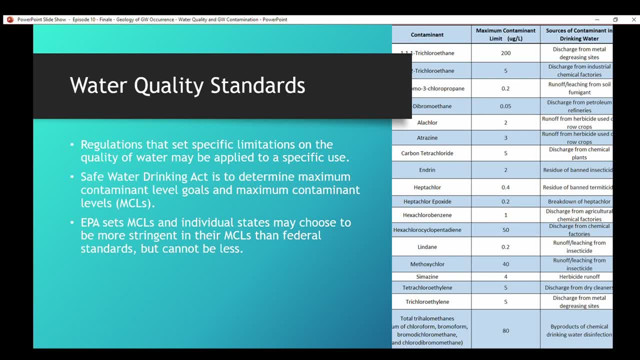 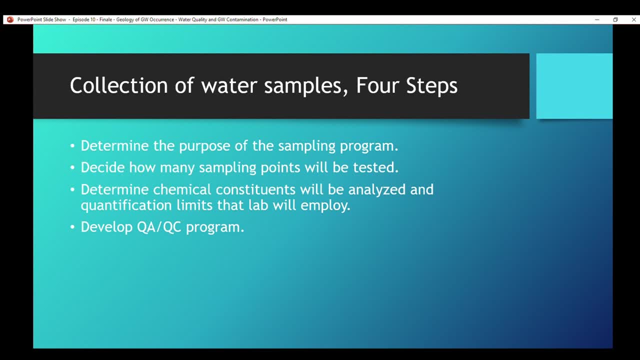 be less so the collection of water samples. there's four steps: determine the purpose of the sampling program. decide how many sampling points will be tested. determine chemical constituents that will be analyzed and quantification limits that the lab will employ. and develop a quality assurance quality control program for your sampling, groundwater monitoring. so determine. 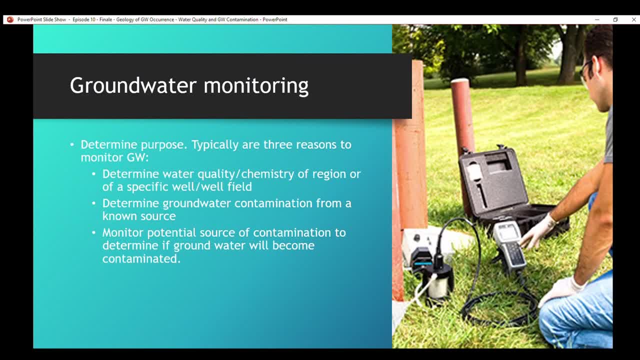 your purpose. typically, there are three reasons to monitor groundwater. so you want to determine the water quality, chemistry of the region or a specific well well filled, which is typically what we do. determine groundwater contamination from a known, known source. that's what we do: to monitor potential source of contamination, to determine if groundwater will become contaminated. 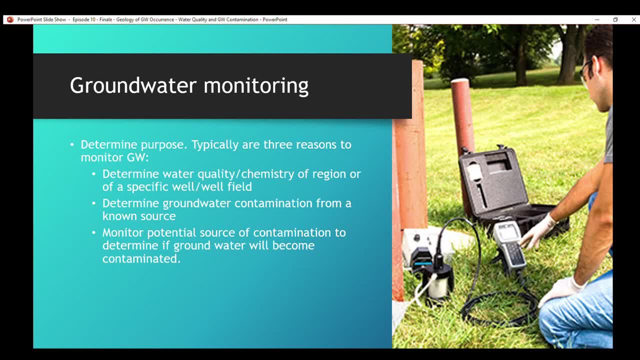 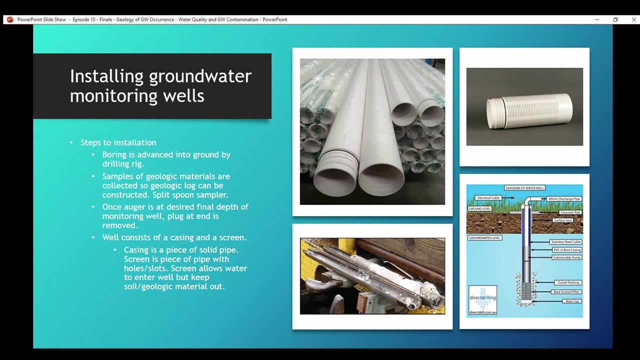 지금은, based on what the test tells you. well, the plug it's plugged at the end of the it's. the plug it at the end is removed, sorry, and the well consists of a casing, which is which is this piping? we typically? I've seen PVC pipe. you can use steel pipe too, so it's basically just. 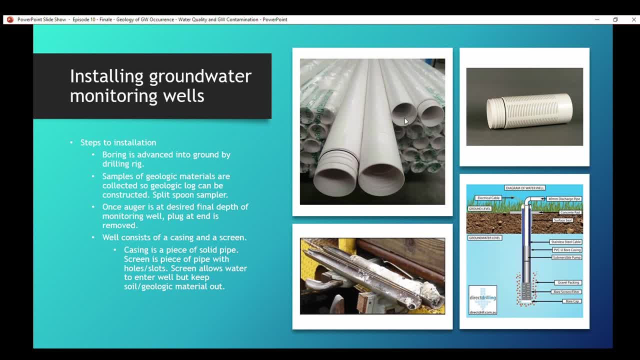 solid PVC pipe. when you think casing and then the screen, is this right here and it has these slots which allows water to, and this is at the bottom of the well. it allows water to go in. it doesn't allow sediment to go in soil or geologic. 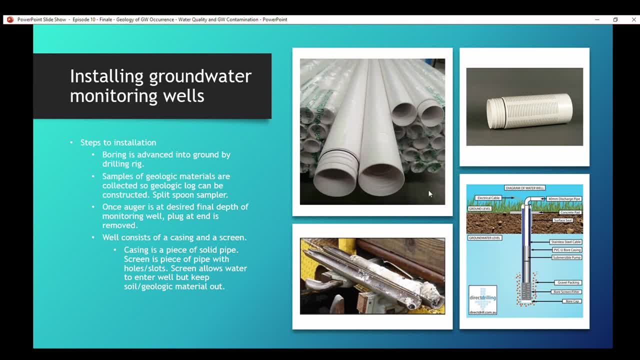 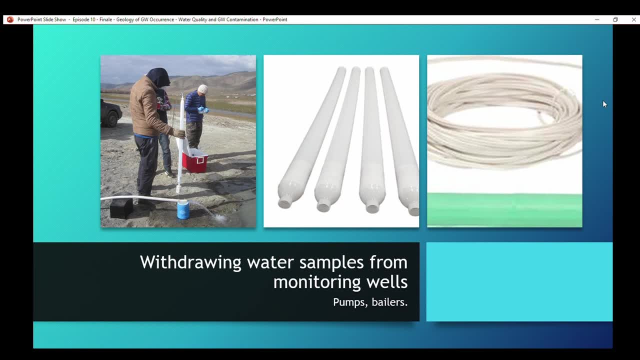 material. you know. so, in terms of withdrawing water samples from a monitoring well, you use a pump or a baler. so a baler is this long white tube. I typically use those if a well goes dry on me from pumping on. this picture got screwed up right here. that's supposed to be a mini. 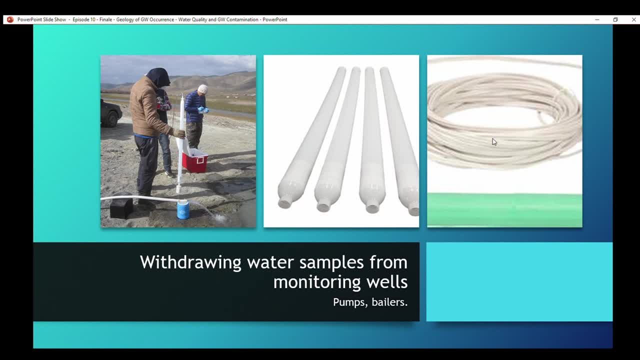 monsoon pump. we use mini monsoons to pump the well and a baler. I typically use it to collect a sample if a well goes dry, or yeah, I mean that's what we do, we. we use these to collect samples and you obviously don't cross. 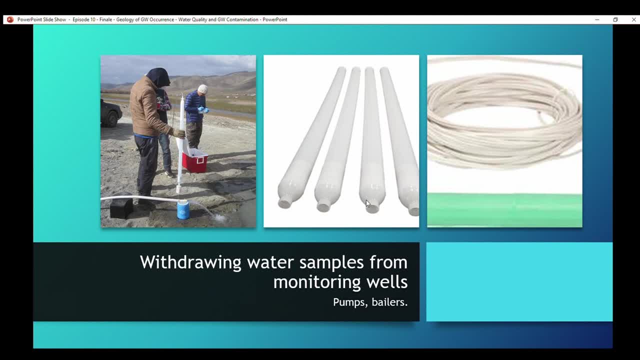 contaminate. between the wells you use a new one for each well. but I thought this was interesting. this has a filter. it's a baler but it has a filter on the bottom, so there must be a lot of sediment in this well that could affect. 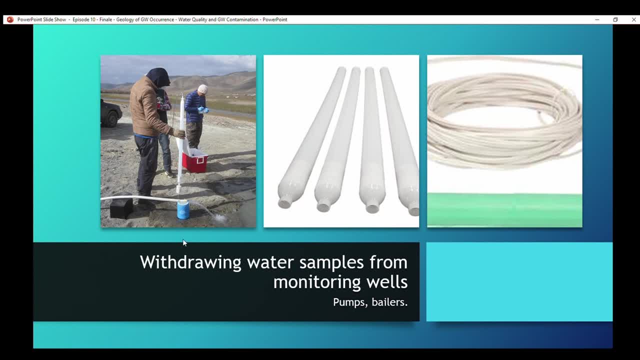 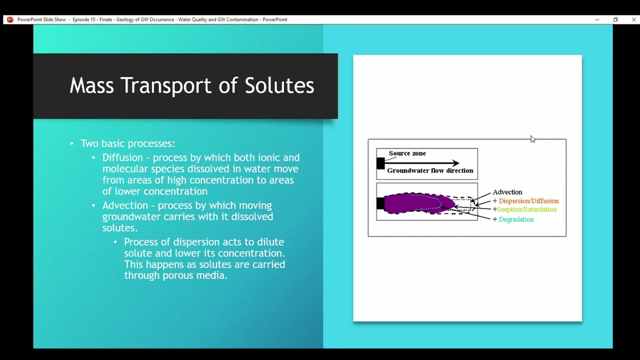 the readings performed by the lab. and then the mini monsoon is used to purge your your wells. sometimes you have to purge 80, 90 gallons out of a well. sometimes it's only like three gallons, depends on the saturated water water column. so, mass transport of solutes. you have two basic processes. 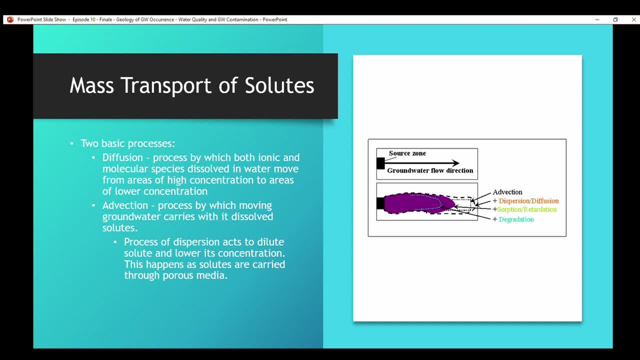 and, yeah, this is a this can get pretty complicated, this process describing how I don't know a contaminant of from a leaking septic tank, how it will go through and spread, and you have two basic processes. you have diffusion process, by which both ionic and molecular species dissolved in water. 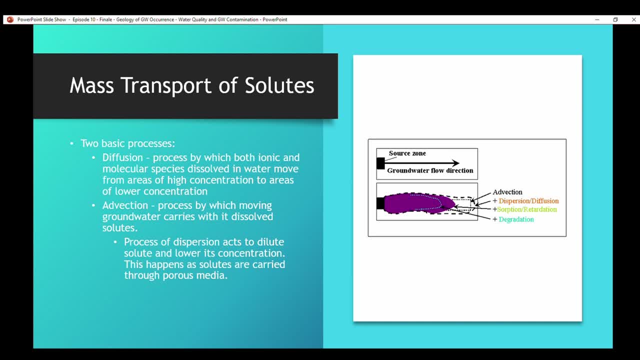 move from areas of high concentration to low concentration. add vection is the process by which moving groundwater carries with it dissolves solutes, and the process of dispersion, which is included in advection, acts to dilute the salute and lowered its concentration. this happens as solutes are carried through porous media, like we were talking about earlier. 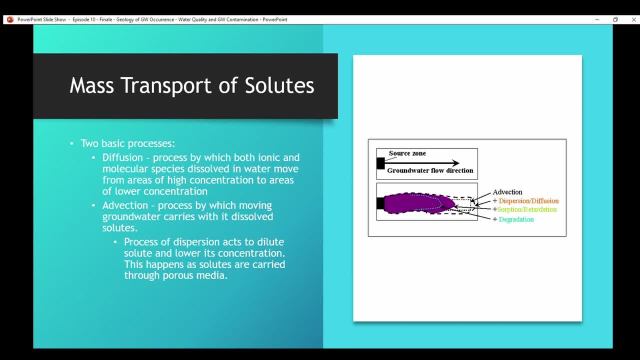 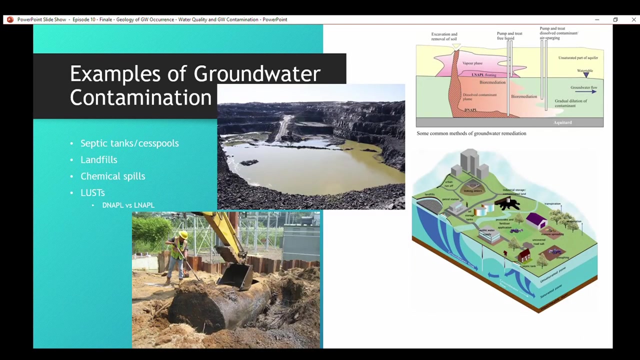 unconsolidated aquifer will kind of act like a filter and you know, some viruses and some bacteria will be left behind as the the contaminant is traveling. the salutes are traveling through the geologic material. so here's some examples of groundwater contamination. you have septic tanks and cesspools. this diagram: 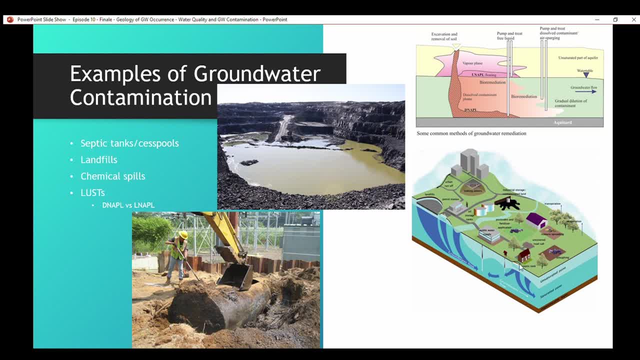 is a good way to imagine. you have a leaking septic tank. it goes into the groundwater. that's bad stuff. landfills they typically. typically you want to have a landfill lined with a shell or an impermeable material to make sure that you don't have leachate entering the groundwater, because 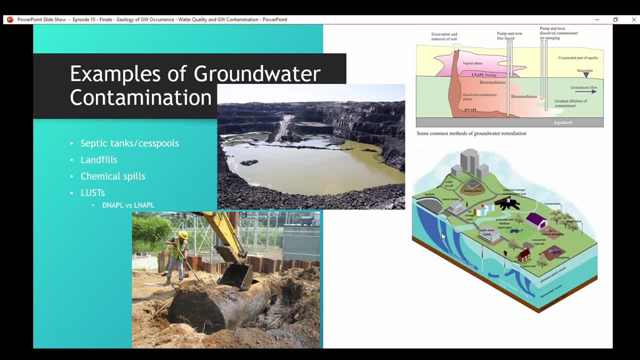 landfills can be obviously pretty nasty chemical spills. let's just look at this one. it looks like oil spilled out of this container and it's probably gonna seep into the groundwater. and it's probably gonna seep into the groundwater and it's probably gonna seep into the groundwater. 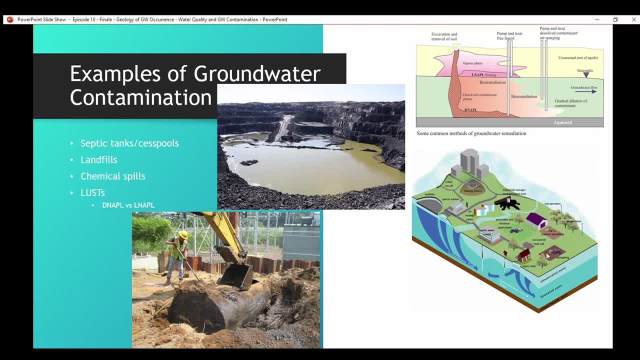 depending on how much spilled out, and then an important one, when you're gonna work in environmental consulting- is leaking. you leaking underground storage tanks and you have what's called dense non aqueous petroleum liquids, and then you have light non aqueous petroleum liquids and basically what that means is this: shows it right here: line Apple will float above.